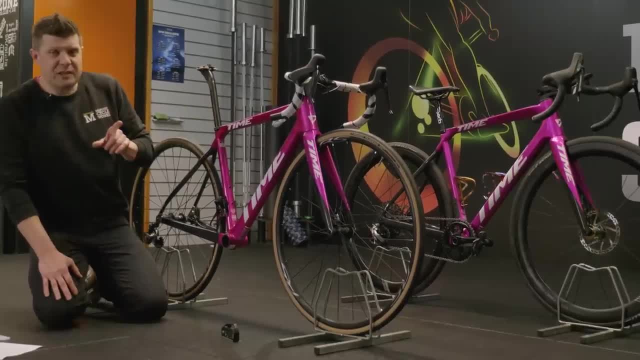 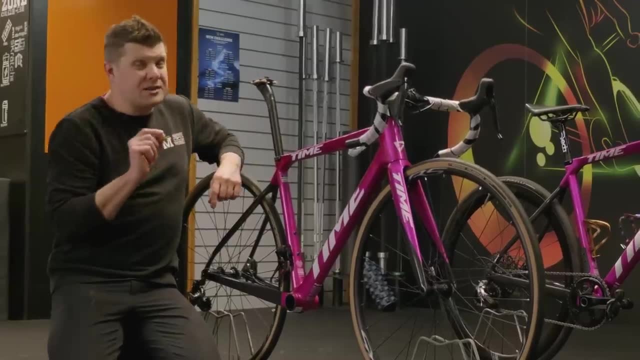 above the bike. could you comfortably stand over the bike? And there is actually quite a big difference between these. It's actually about four centimetres. This is between the top tube here and your crotch. That might be one major pure safety concern. So after that we have to think. 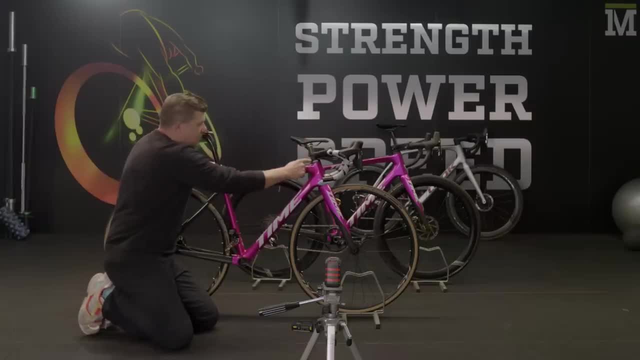 about the length, and you can look at this in two ways: Either the top tube length or the actual reach measured from the bottom bracket. And both of these bikes are actually very, very similar. In fact, if we take a look at the geometry chart here, the distance in reach is only five millimetres, which is next to nothing. 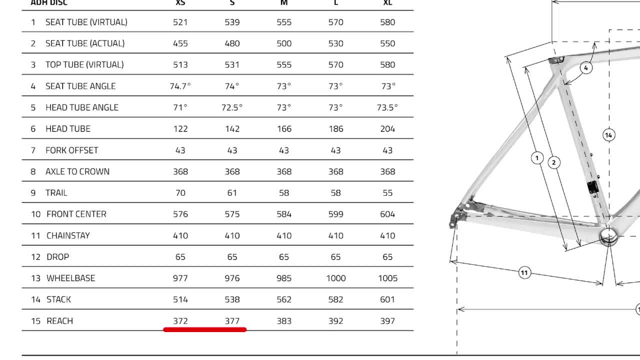 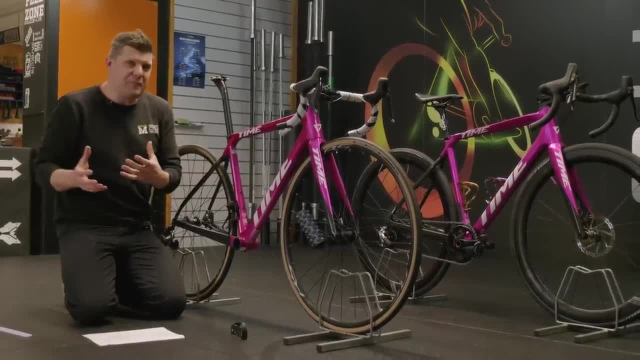 especially when you consider that stems get measured by the centimetre. And that almost has to be the case because, like I say, you have to try and have a sufficient wheelbase that the bike doesn't suddenly become really, really twitchy in handling. 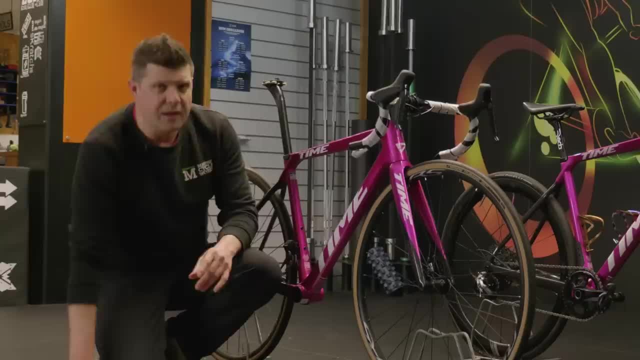 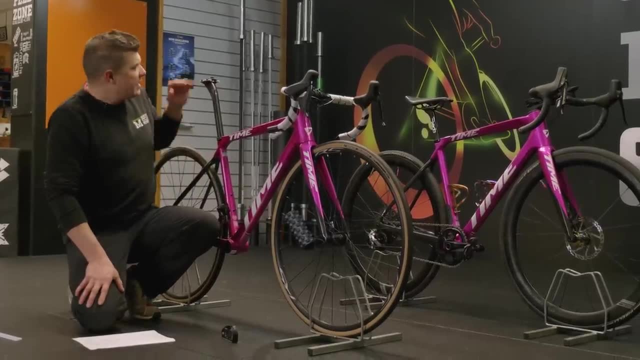 or you end up with toe overlap and all sorts of messy stuff going on. The other thing that can't really change that much is the height of the handlebars, which is where smaller riders really, really struggle, because the saddle to bar drop, that is the distance between the saddle. 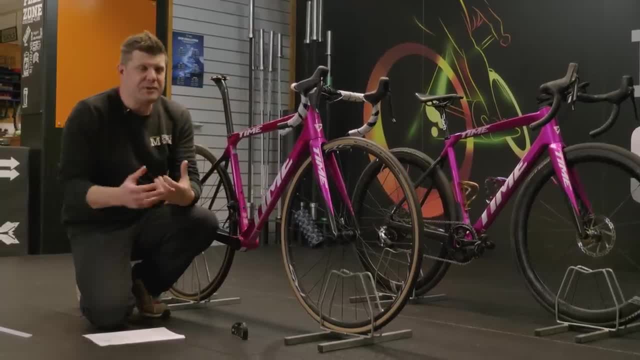 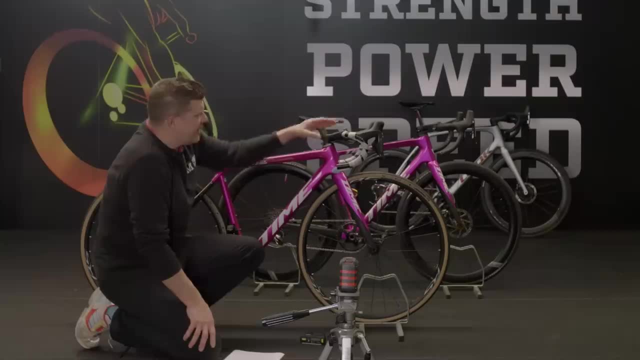 and the bar height here isn't actually that extreme, which means that smaller riders really struggle to get into a really powerful riding position where they can really use their glutes to push hard on the pedals because the handlebars naturally have to be so high to accommodate. 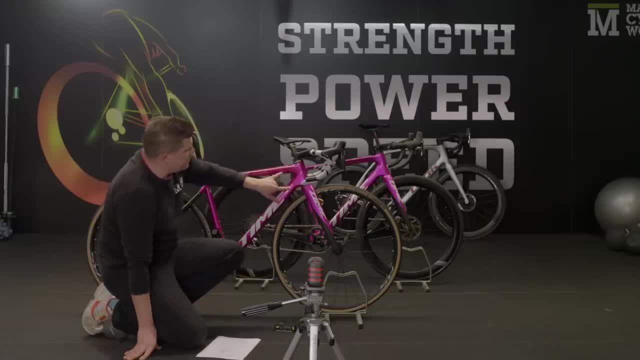 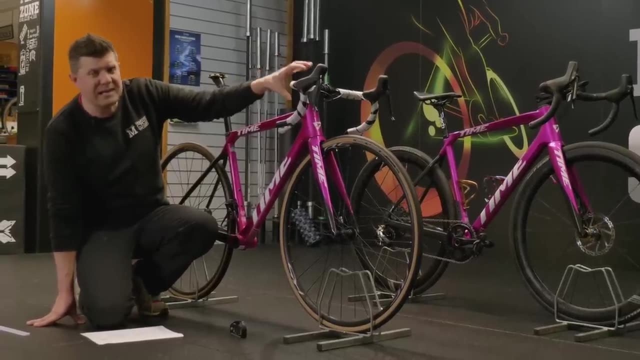 the 700c wheel, the fork, enough of a head tube that the two tubes can actually join, And then, of course, the stem height as well. So you're already restricted. even being completely slammed, you're already at a fairly high saddle to bar drop, One of the very first things you'll. 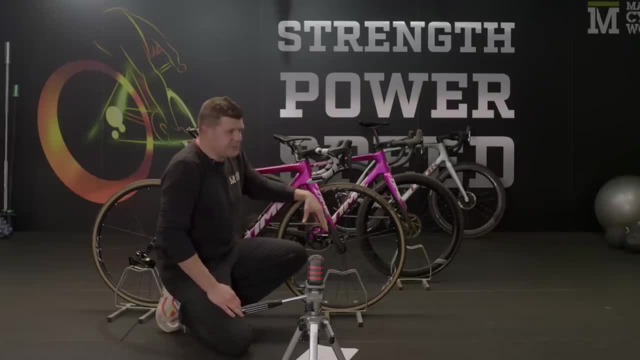 notice when you look at an extra small bike is this angle here seems so much further forward, what we would call slack, and that's in order to make sure this wheel has this space here that we were talking about earlier. Now, this has loads of implications for the handling, and if I was just 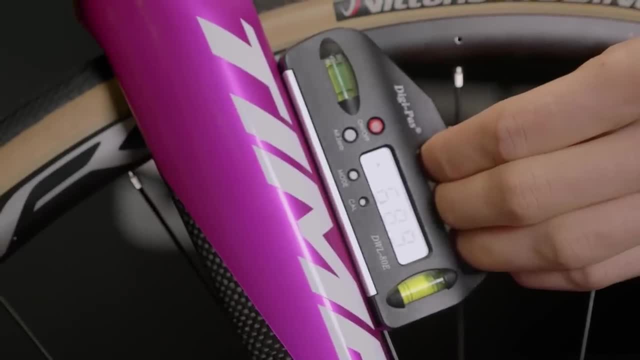 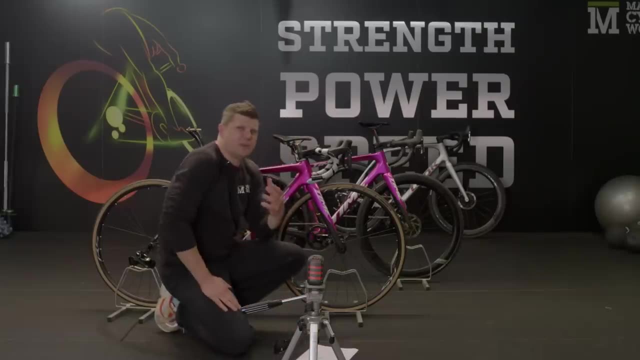 to take our inclinometer and measure this, this actually gives us an angle of around 66, but combined with the angle here, gives us that 71 degrees, which is almost two degrees slacker than the 73 degree angle actually intended for this design of frame. So if I just look at the angle, 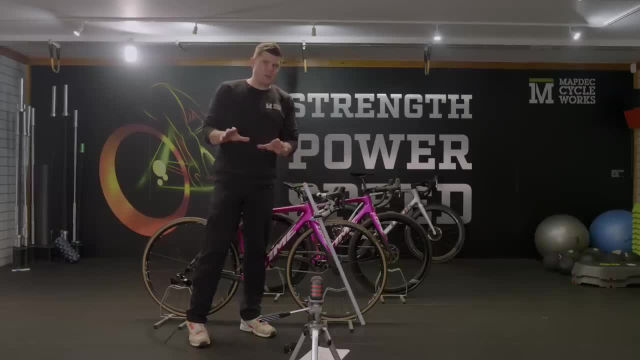 and lay this ruler up against here. it really exaggerates the angle that we're talking about Now. this is going to have quite a big impact on how the bike handles. You see, with the normal 73 degree angle you expect to have that really tight cornering feel that you expect from a race bike. 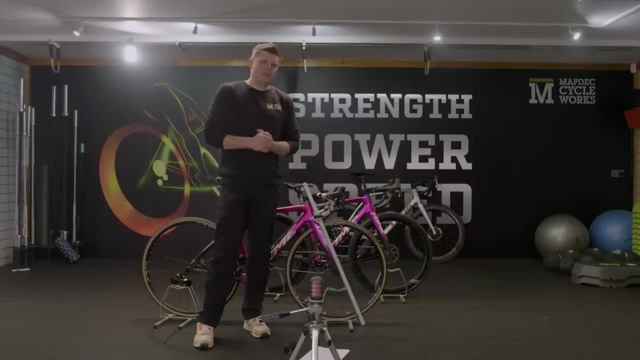 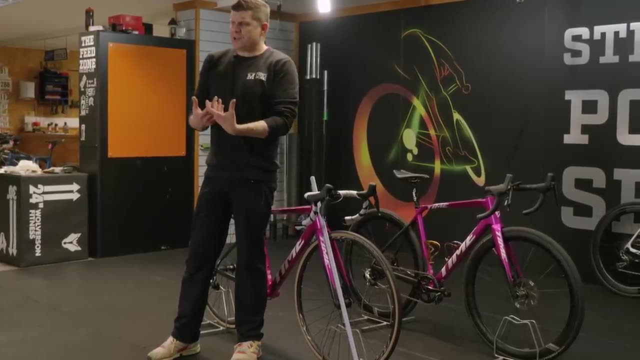 throw it into a 90 degree bend, lean over and really nail that corner. In contrast with something with a slack head angle like this, it's going to handle much more like a mountain bike, which means that if you're rolling in a straight line and you hit a really rough potted road, this is actually 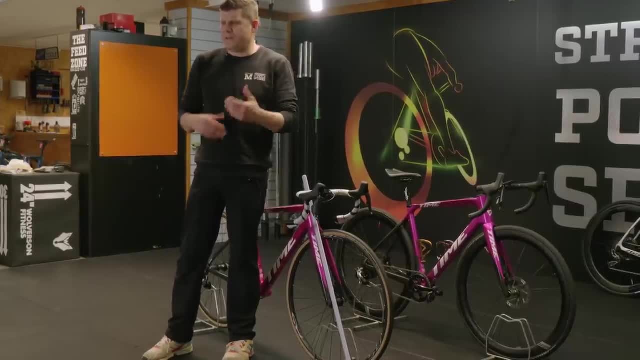 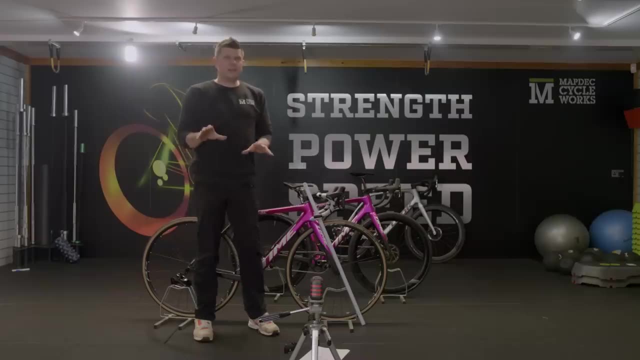 going to feel a lot more stable. when you're going fast. in a straight line It's going to feel like the wheel is going to track over obstacles a whole lot better. but at slow speeds it's going to feel a little bit wobbly. So quite often choosing. 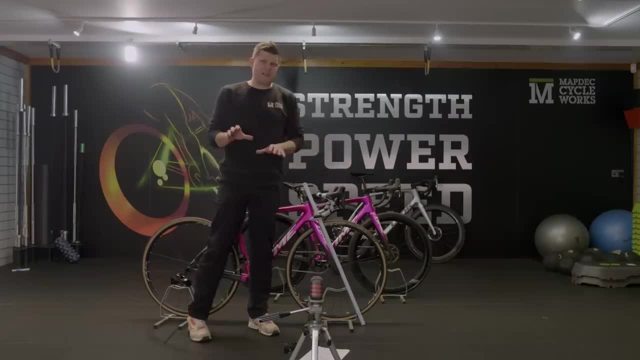 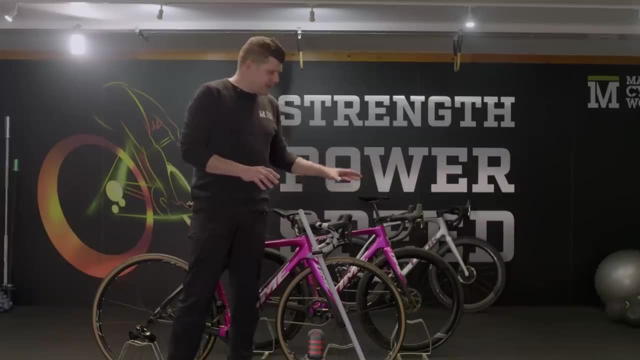 between a small frame and an extra small frame actually comes down to the handling characteristics and whether you want something that's going to feel a bit more racy and nimble, or whether you're doing more endurance rides and actually having a slack head angle more akin to an endurance bike. 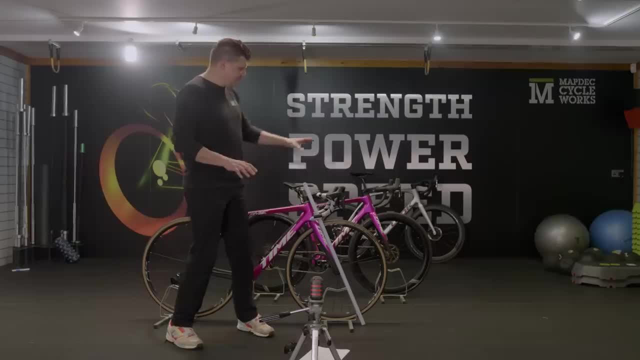 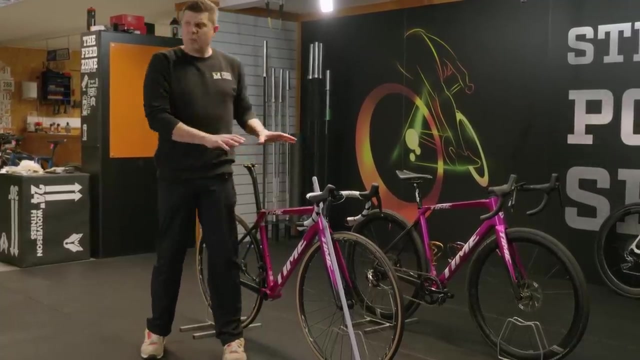 is actually what you're looking for. That definitely happened in this case, because this particular customer said: well, actually I spend a lot of time in the mountains and I really want to feel confident at speed descending steep hills, you know, in the rough roads. I said this is the one because your actual position will 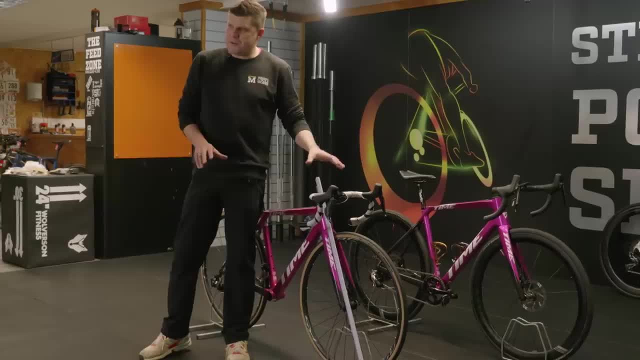 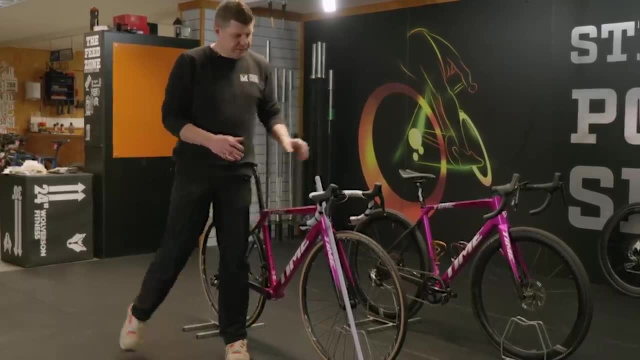 be able to get exactly the same between the two bikes, But this one offers the best geometry for what you're describing without having to go into an endurance bike. gives a really, really nice compromise. I just want to reiterate the point that how difficult it can be to buy a really 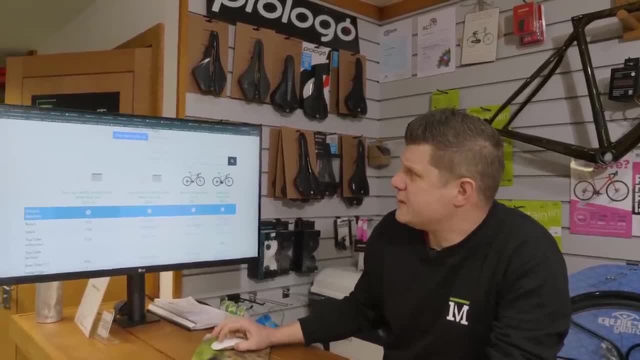 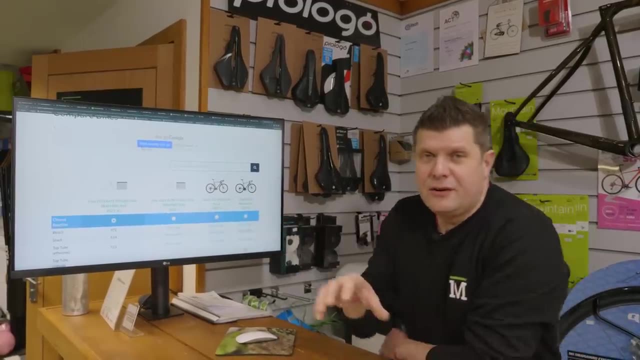 really small bike. So this is the Geometry Geeks website. I've just pulled up the two time bikes that we're looking, and I've also pulled up the Giant TCX and the Giant Defy. Now you guys often ask me why I always pick on Giant. Well, there's one simple. 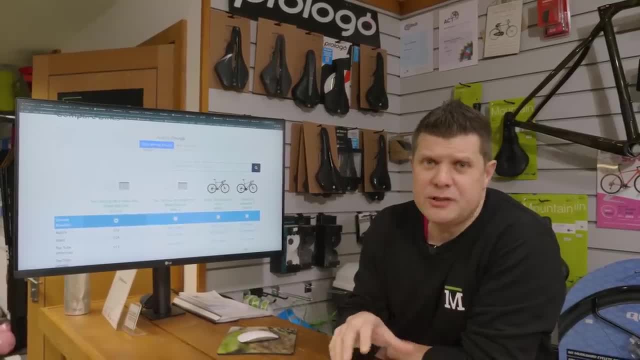 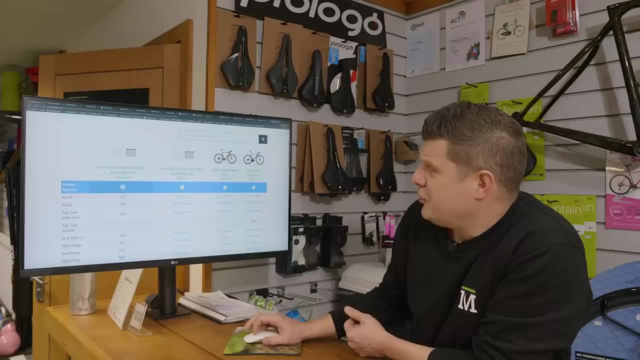 reason: It's the biggest bike brand in the world. They're absolutely global. Everybody watching this video has heard of the Giant TCR and the Giant Defy, So it makes pretty good sense just to compare them to lots of different things. So this is the crazy thing about small geometry, Remember. 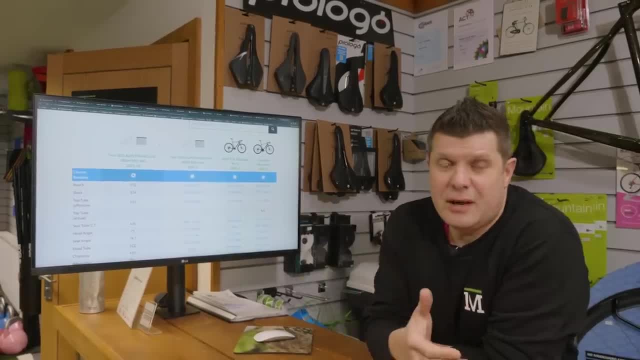 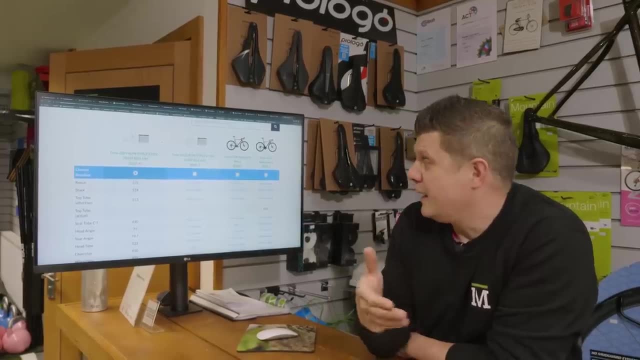 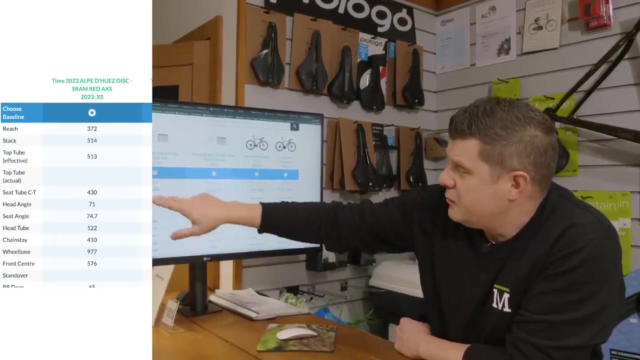 the Giant Defy should be their endurance bike, and endurance bikes typically have a higher slack. a shorter reach and also a slacker head angle would make it an endurance bike. But they don't do an extra small in the TCR or the Advance. You're stuck at a size small, So I've pulled up a. 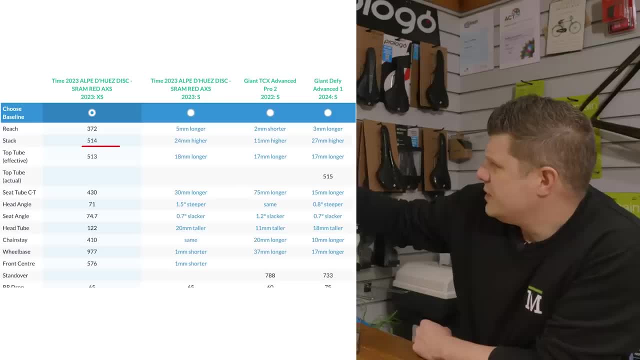 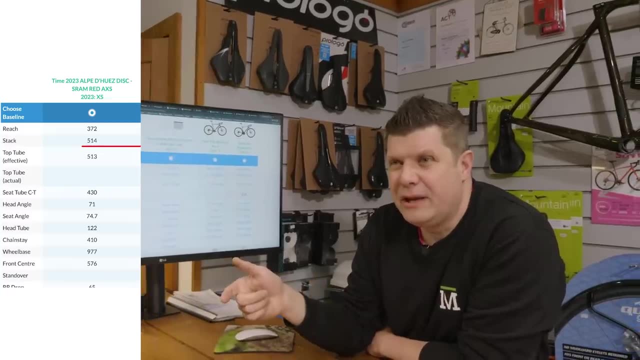 size small here as well, And you can see that the actual, the Giant TCR actually has an 11 millimeter higher than the extra small. Now most small riders actually have the opposite problem. They have the problem of trying to get the handlebars low enough rather than necessarily make them higher, like 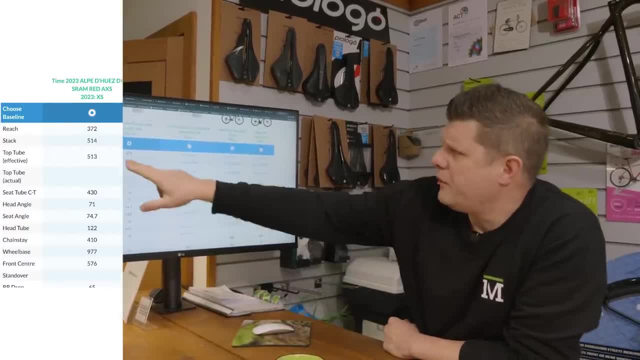 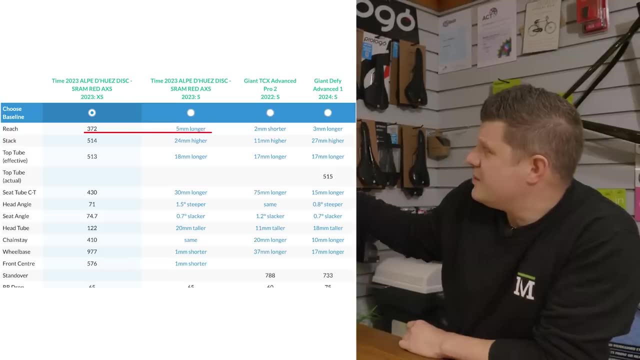 people in the size medium, A size large frame would do. And while we're on this top column here, the reach. this is what most people associate with going down in size, But you'll see that the reach is actually very, very similar, because at some point you can only make a bike so short because you're stuck with the size. 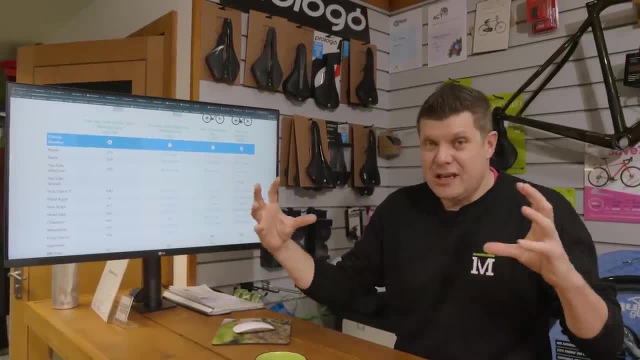 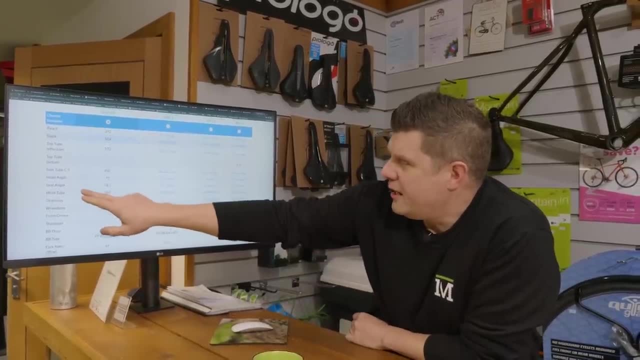 of your feet, the size of the cranks, the size of the wheels, And you can't just keep making things smaller and smaller. So compromises have to happen somewhere, And this is where the compromises normally happen is down here, on the head angle and the seat angle, And most of the time when you're 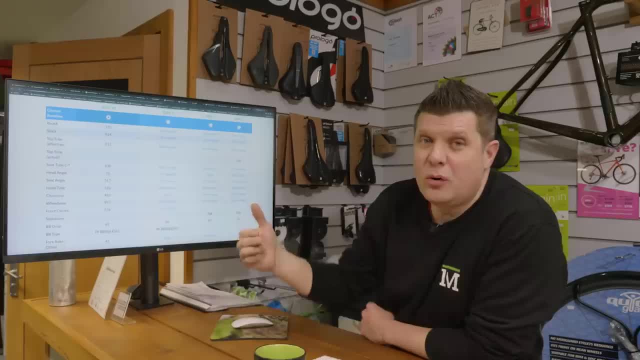 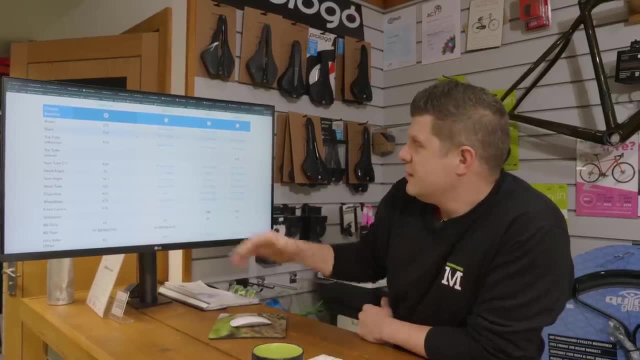 looking at an extra small or a small bike, you're going to have to make sure that you've got the right size of the bike. You'll find that you're already riding what would essentially be endurance geometry for a person riding a medium or a large frame. So when you see an endurance bike in a 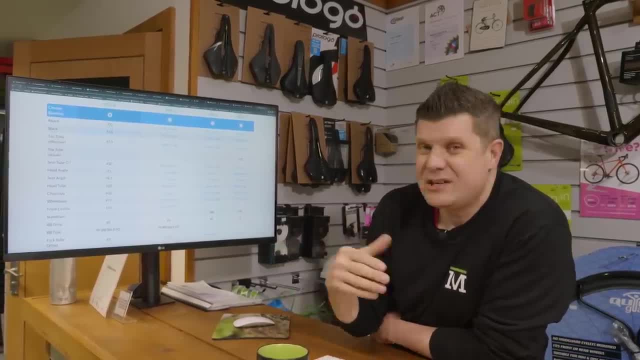 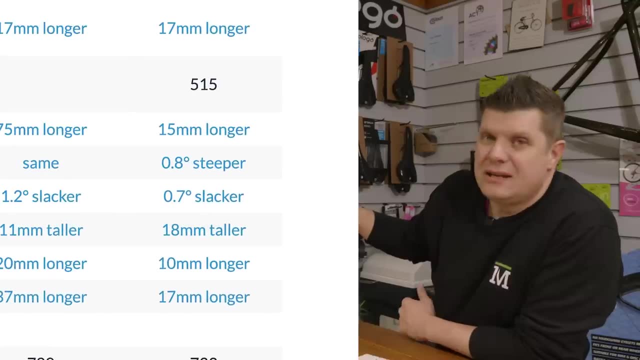 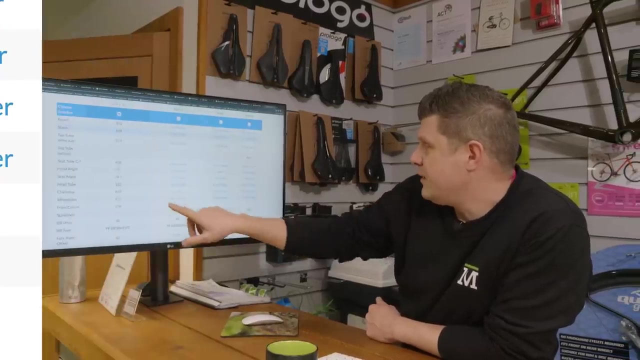 small size that just gets exaggerated more and more and actually some really, really funky things start to happen. So you can see here on the Giant Defy that the head angle actually gets steeper And that's because the wheel base here has got significantly longer, And they've done that. 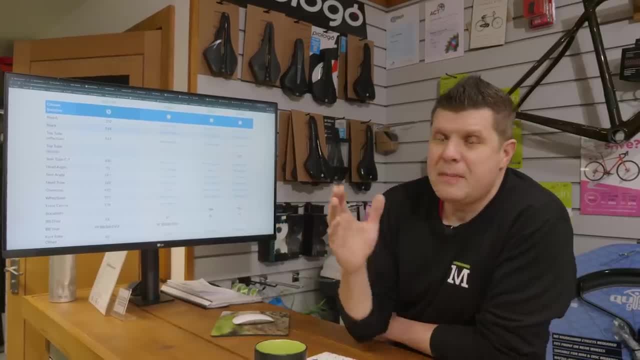 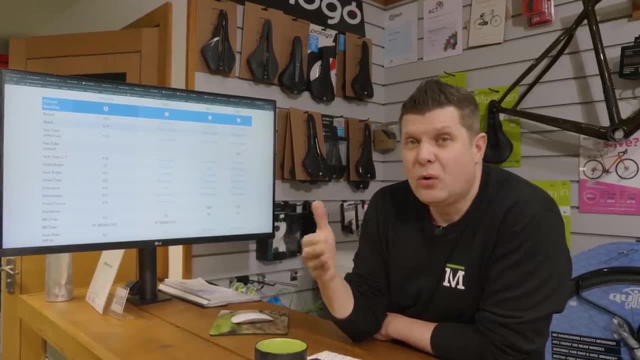 making the chain stays quite long as well. so by making the chain stays longer, you stabilize the handling at the back, but you also take away some of the nimble cornering abilities as well. so it's not always a good thing just to keep making things longer and longer. the point i'm trying to make is: 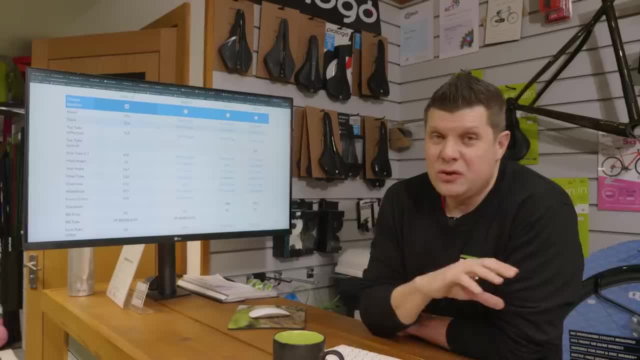 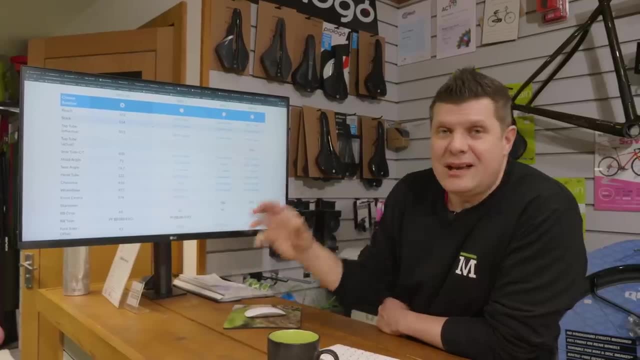 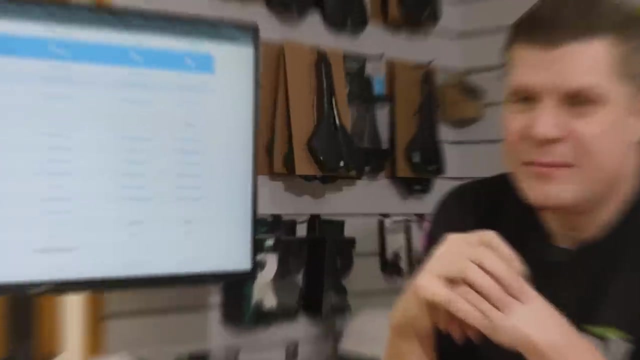 when you're buying a small bike or an extra small bike, you've got to put way more thought into it than just does it fit, because there are so many more handling characteristics that go on as brands try and squeeze in wheels and crankset into a smaller and smaller package. now, when you're. 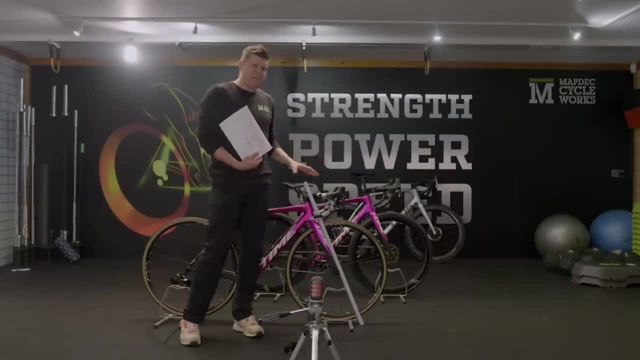 looking at the geometry chart of a bike that you might be interested in, you're going to see this effect described under trail, and trail is the distance between where this white stick is interacting the ground, and if i turn my laser level on here. so what i've done here is moved. 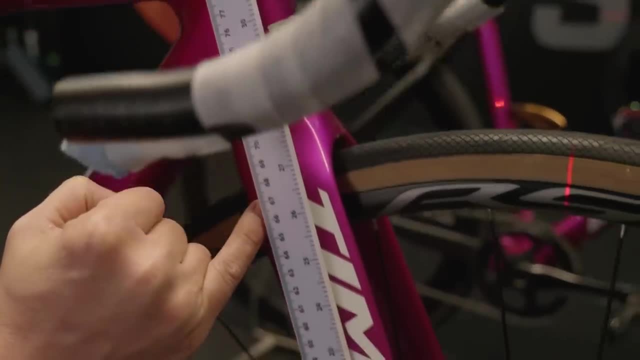 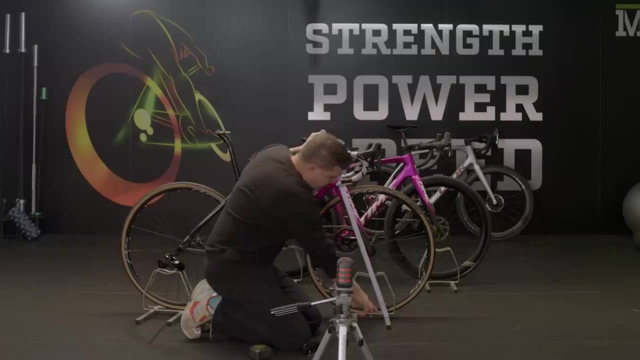 our white ruler to the center of the steering axis. so it's taken a line here through the center of the steering axis and this red line is demonstrating where our tire actually touches the ground. and the difference between these two marks here is what we call trail. now on here is actually quite 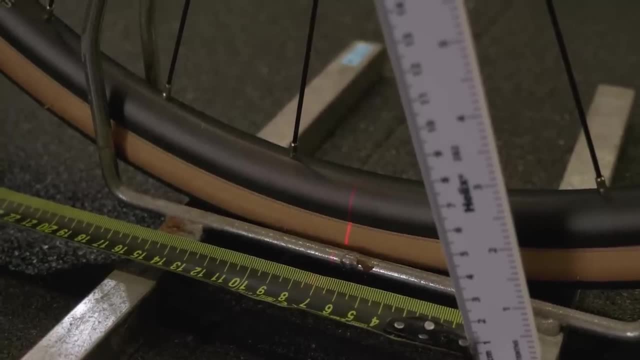 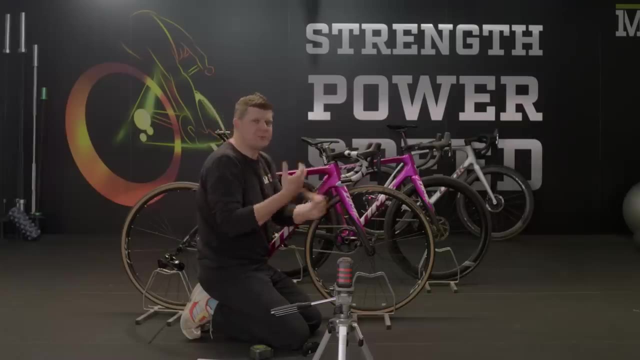 a long trail. it's almost seven centimeters, which again almost puts you into mountain biking time trial sort of territory where you need your front wheel to be very, very stable as it's hitting obstacles or you're in a more compromised position. doesn't necessarily lend itself into nimble. 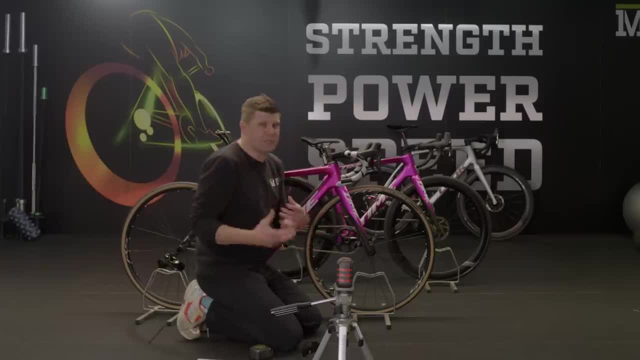 handling, i throwing it into a corner and adjusting your weight position like you would do in a road bike race. now, this is probably the biggest difference between these two frames because, looking at the geometry chart here the size small has a trail of 61 millimeters, compared to this one at 70. 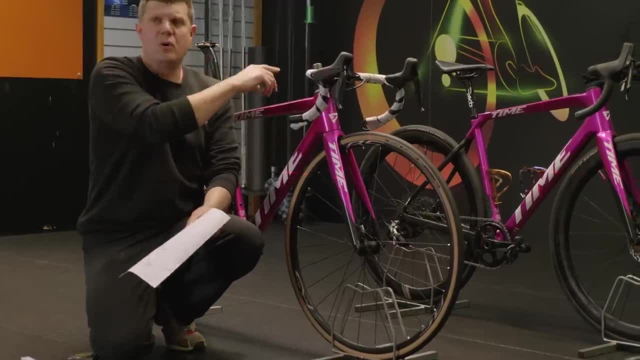 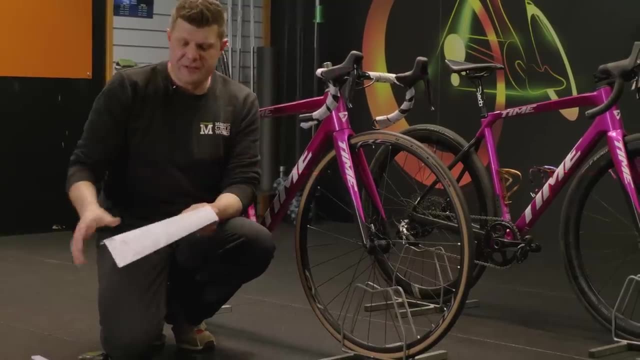 that's a nine millimeter difference now compared to that small on the medium and the large, which were designed around a 58, and therefore only a three millimeter difference. the jump between a small and an extra small when it comes to that trail measurement is absolutely massive. so there's. 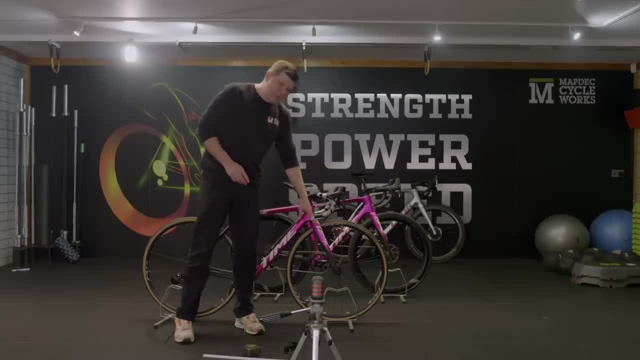 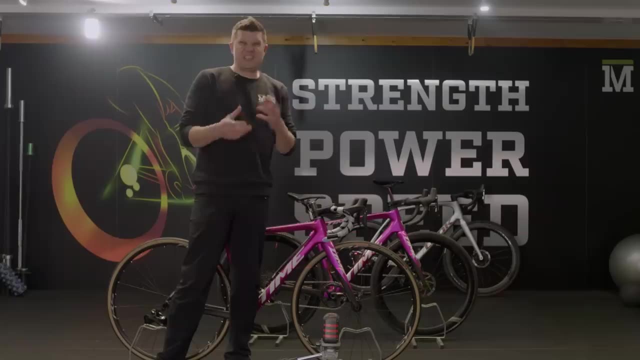 one more thing to consider while we're up in this area, and that is with this slacker head angle. we also have the problem that our stems don't come in at an angle that we want to be able to use, the angle that corresponds. normally, the stems come with a six or a seven degree angle to correspond. 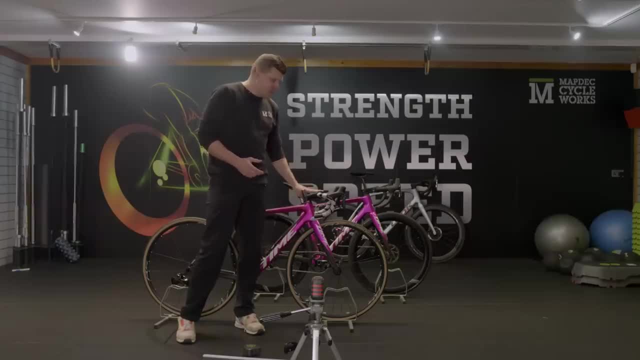 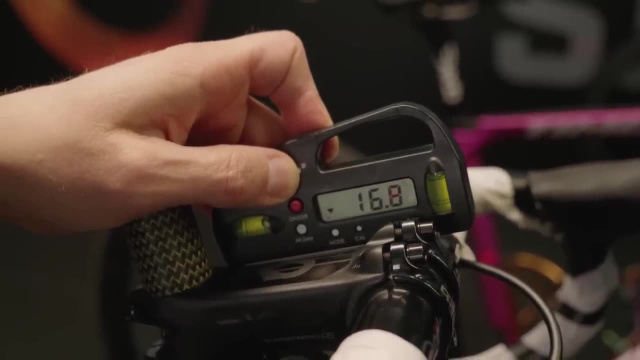 to the 73 degree angle of our steering, which means that we get this nice straight angle, with this being slacker. it now means that our stem now has a slight positive angle, which means that our handlebars are higher, which again is that problem that we have with smaller people not being able. 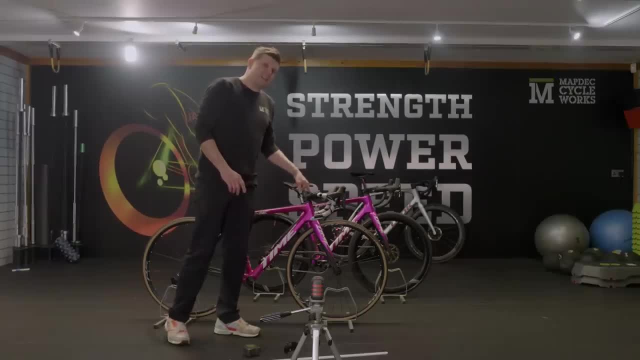 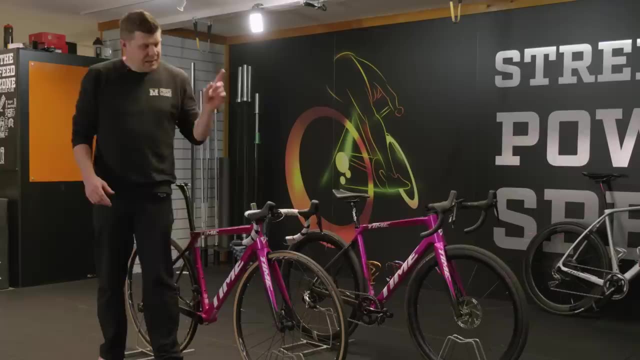 to get the saddle to bar drop so you can actually get stems which are more of a negative rise. maybe it comes down to a minus 10 and minus 12, even minus 20.. however, if your handlebars start to go below this, bearing with a really negative stem, then you have other. 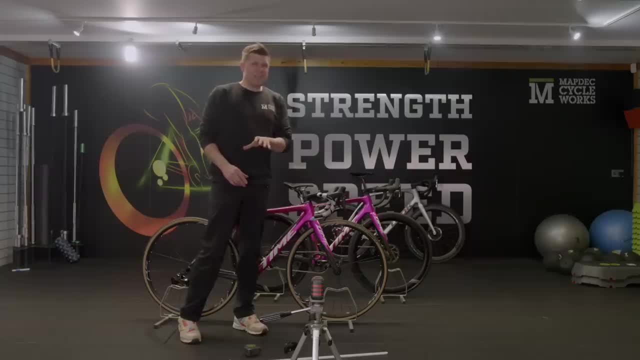 handling considerations to think about as well. you don't tend to see this that much, maybe on a few time trialists, maybe you sometimes see it on a world cup cross-country type bike, but for most road bikers they tend to keep the handlebars at least level with the top bearing. one more important: 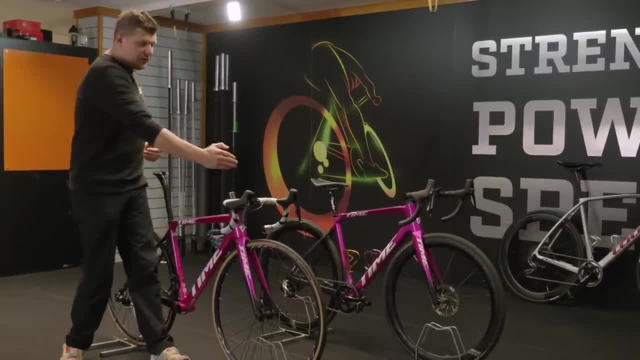 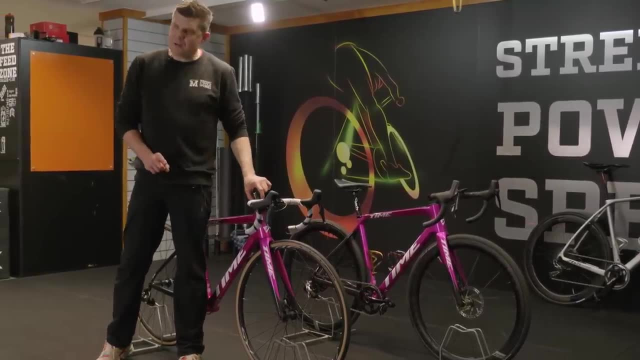 note about stem length for this. if you really are struggling with the actual overall reach, you need your handlebars to be that much higher than your handlebars. you're going to want to keep the handlebars closer to you. if you put a very, very short stem on a very slack head angle bike, you're going to get 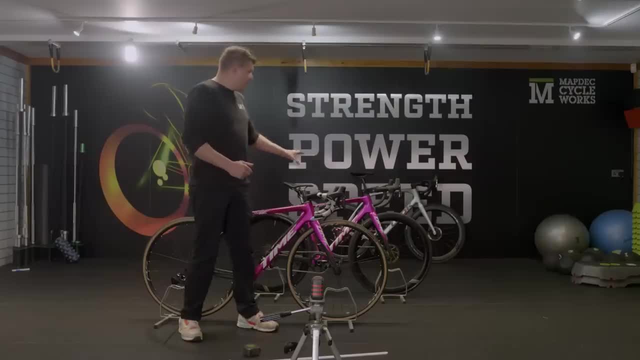 some very funky handling indeed. so sometimes, if you've got the stand over height to do it, you're better off putting a shorter stem on a bike with a more normal head angle than you are putting a short stem on a very slack head angle bike and then try to keep the handling somewhat under. 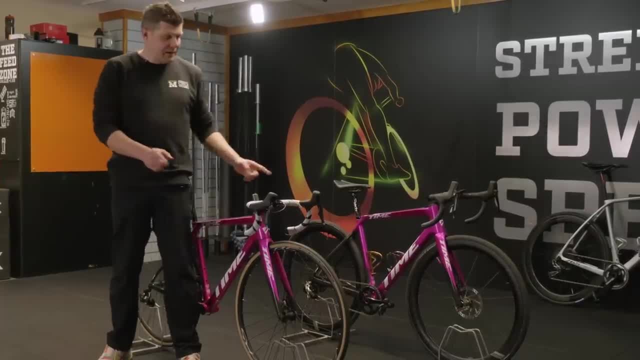 control, especially if you're also running narrow bars. because you have a narrow 38 or 36 centimeter bar and a very short stem, you're going to want to keep the handlebars at least level with the top bearing and then try to keep the handlebar somewhat under control, especially if you're also running narrow bars. 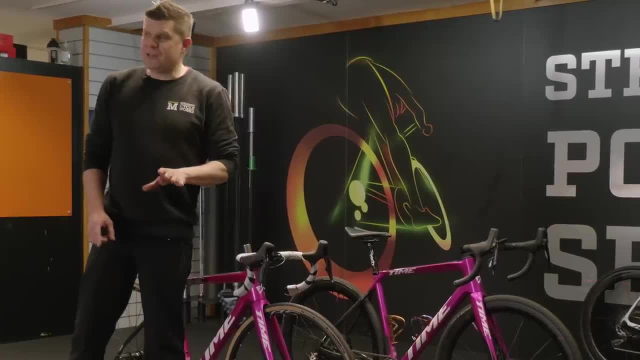 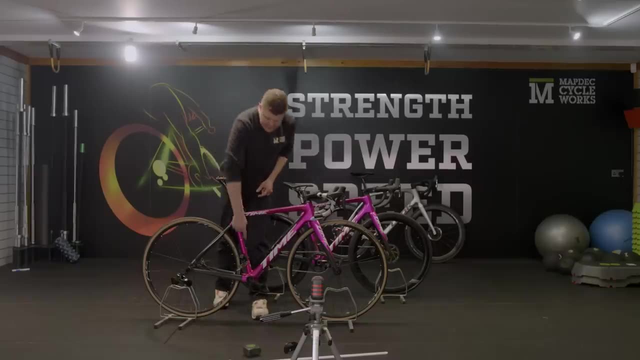 short stem and a very slack head angle, you're going to have absolutely disastrous and scary as hell handling. it won't be a cool ride, okay. the other thing that needs to change on extra small frames is this: this is the seat angle here now, in order to accommodate the rear wheel and make 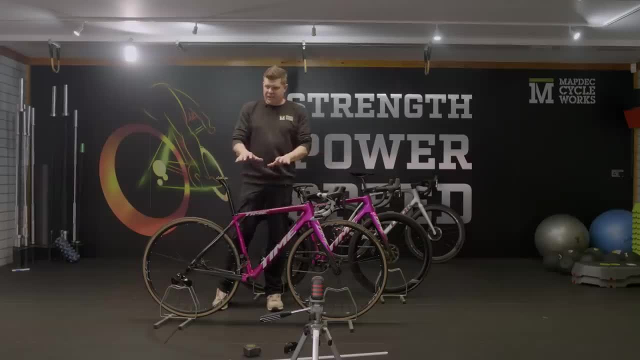 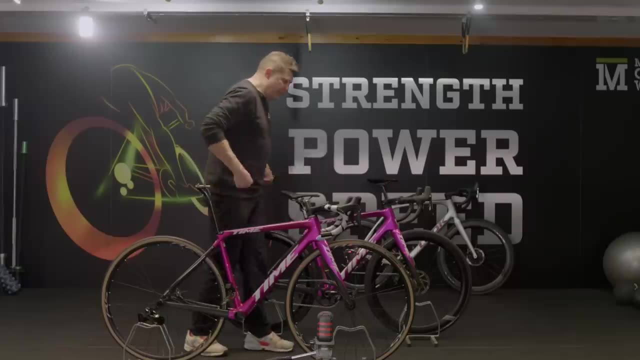 sure that our center of gravity stays somewhat over the bottom bracket. we normally see these get a little bit steeper into a 74, maybe even a 75 degree angle, which means that as you come further forward your hip angle is naturally going to open. now you can offset that by then trying to lower. 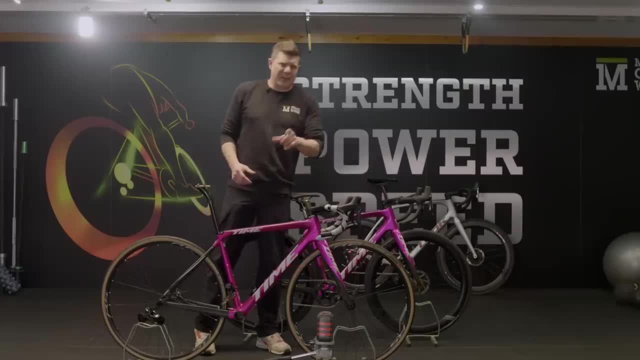 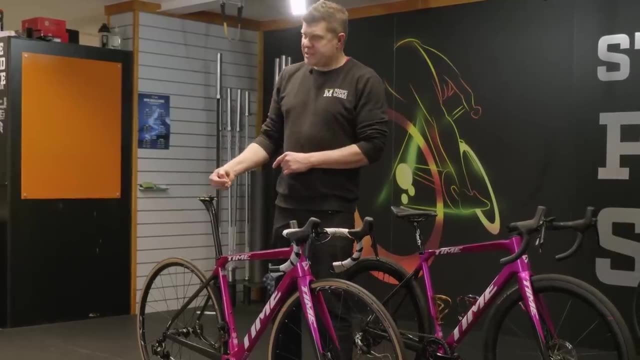 the bars even further, which you'll often struggle to do, like we've just talked about. so you've sometimes got a problem that's a little bit compounded, but what you might find is that by moving this slightly forward, opening that hip, you can actually probably run a longer stem than you. 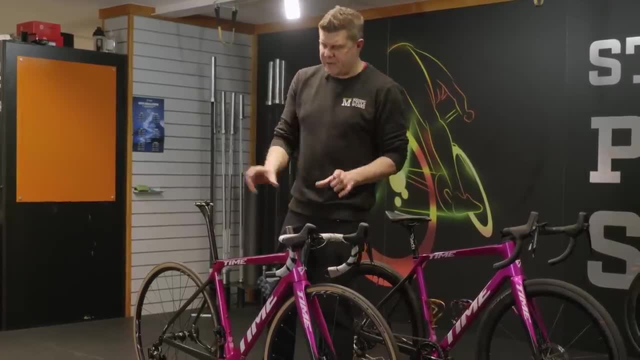 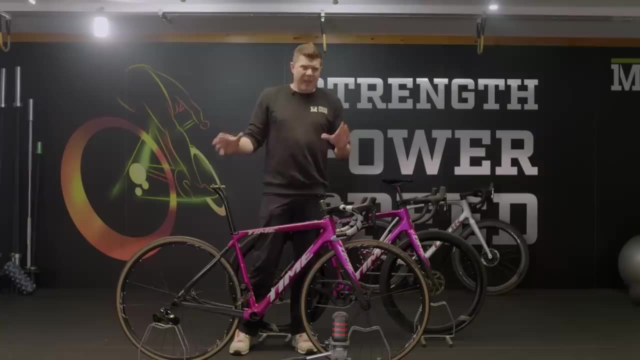 think you can and actually put some control back into your steering with an extra small bike. so, for example, this particular customer came to us with a bianchi that they had heavily modified to try and get it to fit, and they came with a very, very short stem and they're 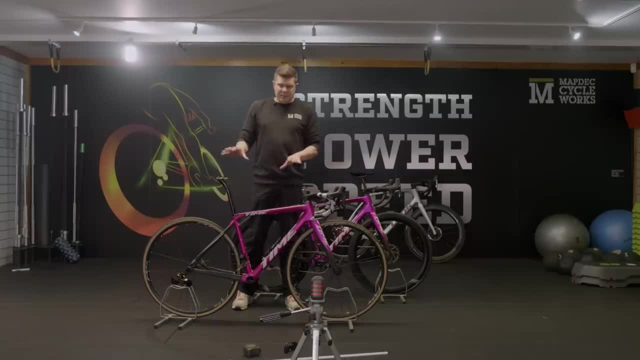 going to try and make sure that the hole this is kind of fits very well and they can lower it down even further and that way you can give them a better foot position and a better steering feel and you can get exactly the same value from the height that these bikes come in. so we've got a 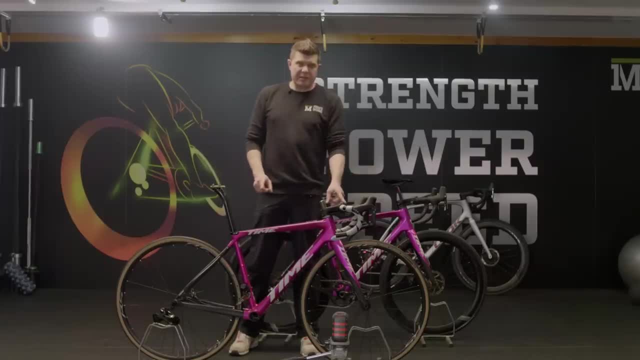 feel and a better try at breaking down the proper height. so once i was done with the front of the, the front of the rails, with the extra small, we can get a better geometry setup for what you want with the extra small than the small, even though i could get the contact points in the same place. 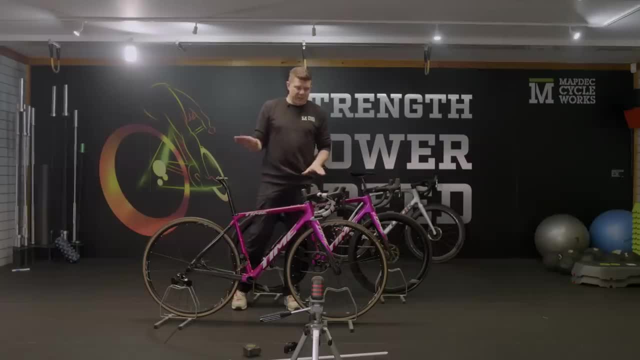 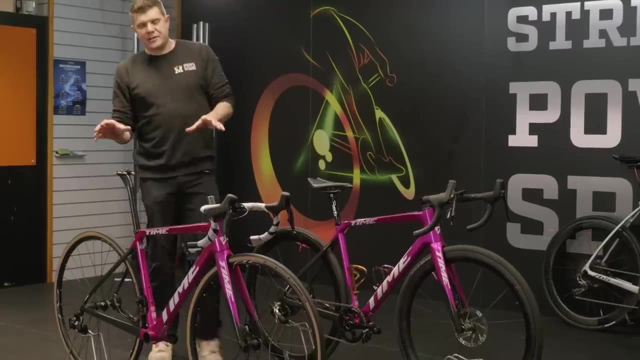 with both these bikes. what this meant was that we could run that slacker head angle. i can run a. in fact i think we might even change the stem and try and go a little bit lower. but we'll find that out when they come for their bike fit okay. and the very last thing, and a bit of a word of warning: 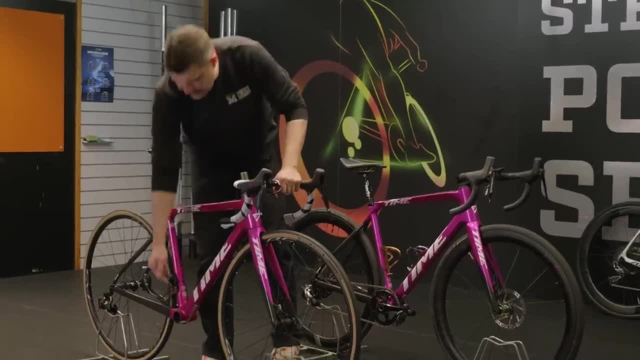 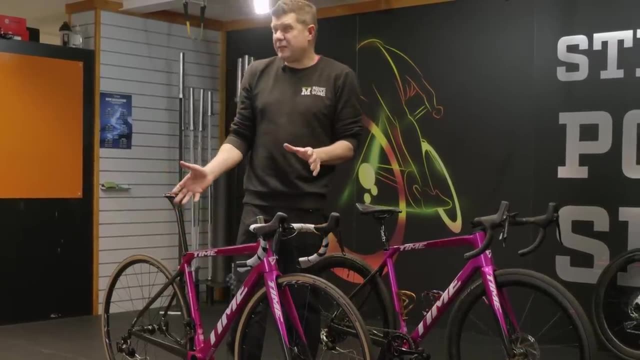 that, as you can see, the distance between the bottom bracket and the wheel gets very, very shortened. so so, if you're buying these off the shelf a few years ago, this would come with a normal 172.5 millimeter crank, and you get all sorts of toe overlap problems, and that's when your 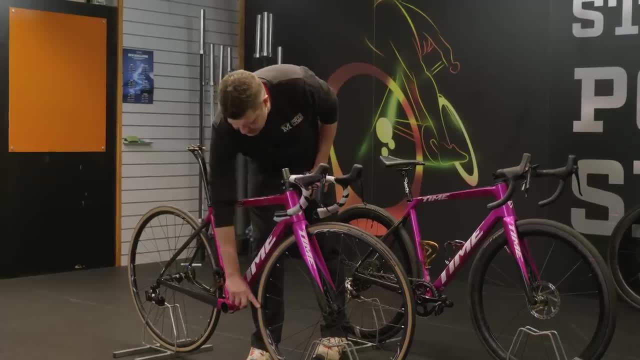 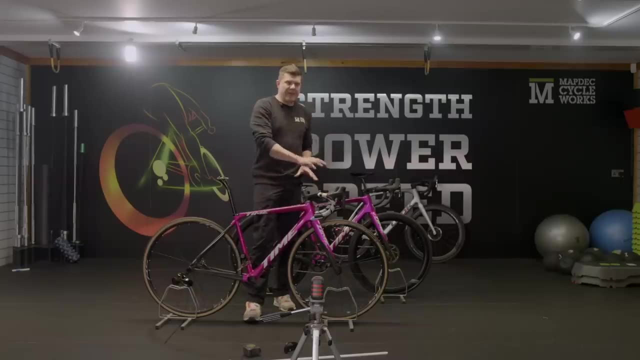 wheel turns here and actually the toe of your shoe will be hitting. it's absolutely terrified if it ever happens to you. but at least for the last five or six years you'll find that nearly every brand has got on top of this and they're now starting to provide shorter cranks. but if you are home building, 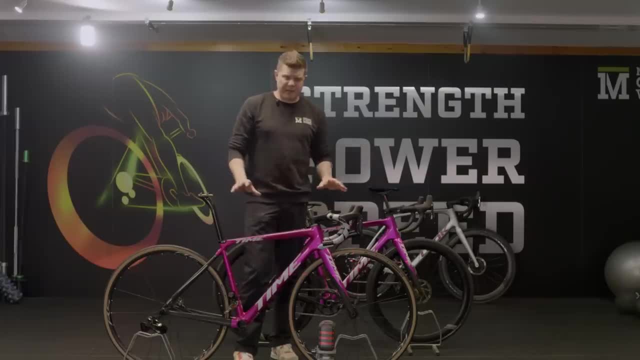 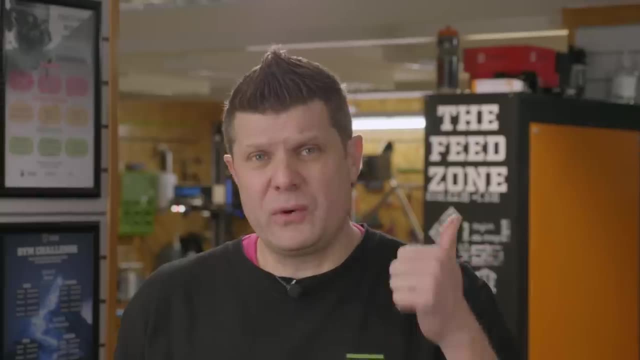 the best thing to do is just go for these shortest cranks. you could possibly find and avoid any sort of situation where that toe overlap is likely to happen. top tips if you are buying a small or an extra small bike. first of all, get the stand over height right, because that might be your. 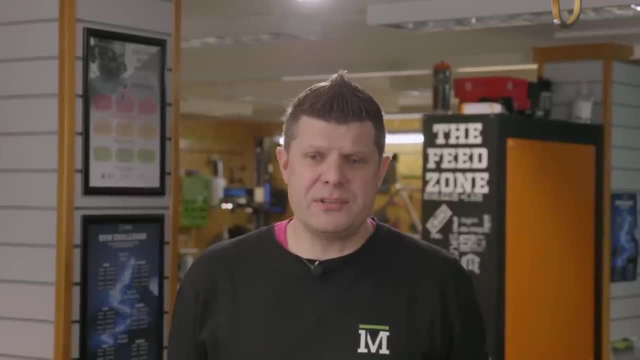 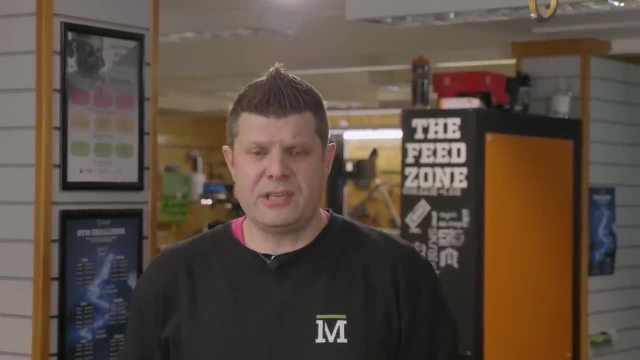 limiting challenge, choice and everything else i've talked about in this video is completely irrelevant. so so long as you can stand over safely a size small or a size extra small, then you can start thinking about the other considerations. so number two: we've learned that the reach is fairly irrelevant. 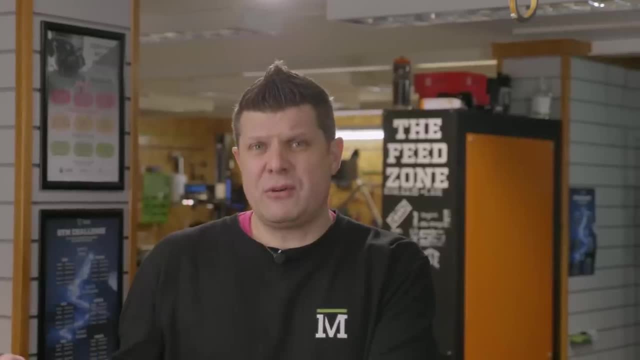 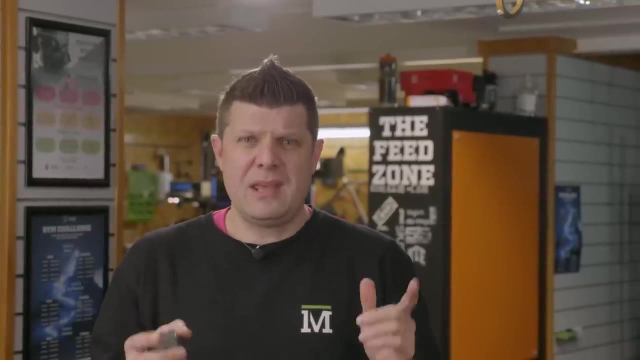 but if you're trying to make something shorter, you might be better off going for a size small frame, because the handling will be less affected by reducing the stem length and your handlebar width. if, however, you can ride a longer stem, be better off going for the slacker head angles that you'll 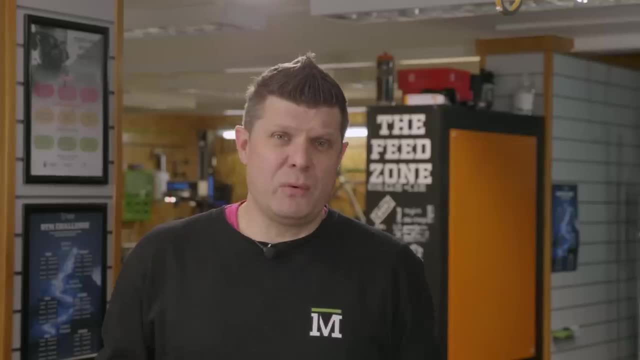 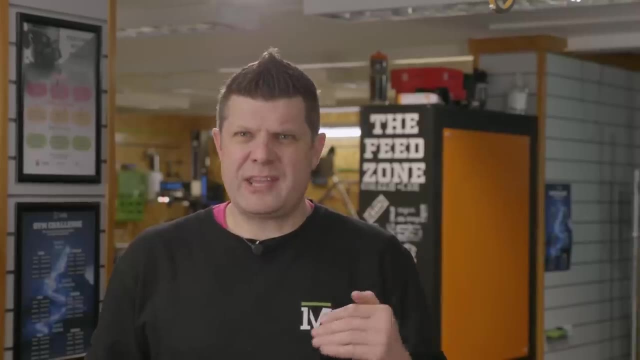 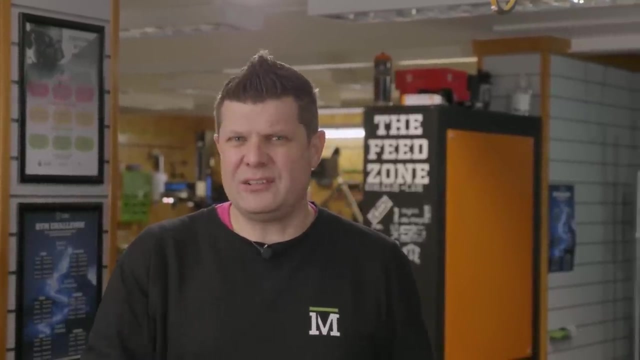 normally find on the extra small frames. tip three: if you are in the fortunate position that you could ride either frame quite happily, then really make sure you pay attention to the geometry and really understand the characteristics found in head angle and seat angle and choose a bike that's going to match the type of riding that you do in terms of its handle in and ride feel. 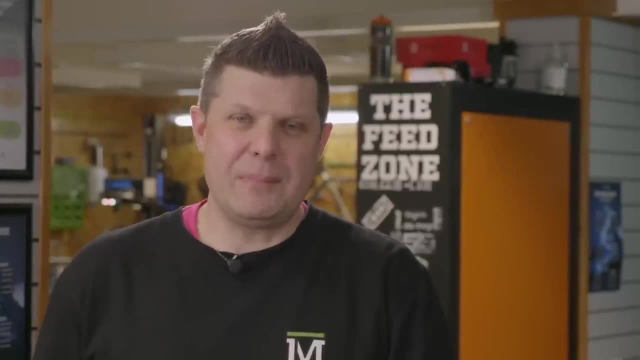 and the last thing, really pay attention to that potential of a toe overlap. just make sure that you give yourself at least four centimeters, probably between the pedal and the wheel, and you should be good. okay, i hope you found that video helpful, if you did give it a rating and. 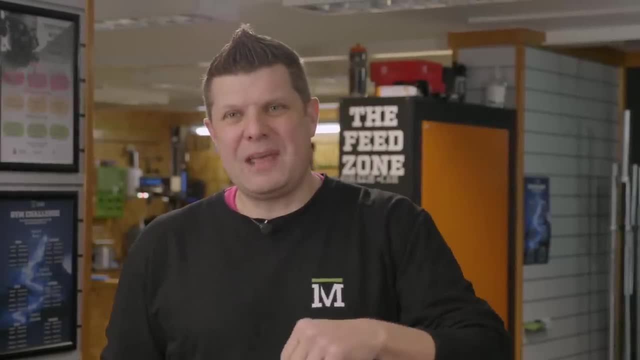 that's what we'll do next week for the next videos. if you want to get ready for the next video- somewhat useful If you did- please get down in the comments and let me know, give it a thumbs up, And if you want more content like this,